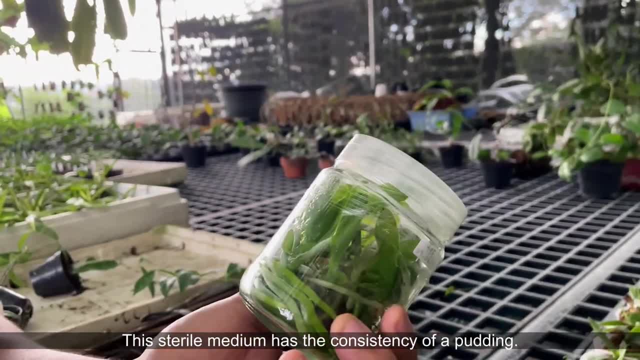 and then I'm going to plant a plant each year. So let's get started. Okay, let's get started Now. so let's start. like pudding. there are grains, there is also nutrition, there are vitamins and so on. 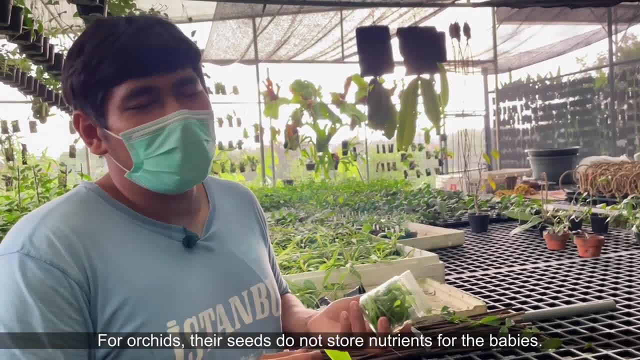 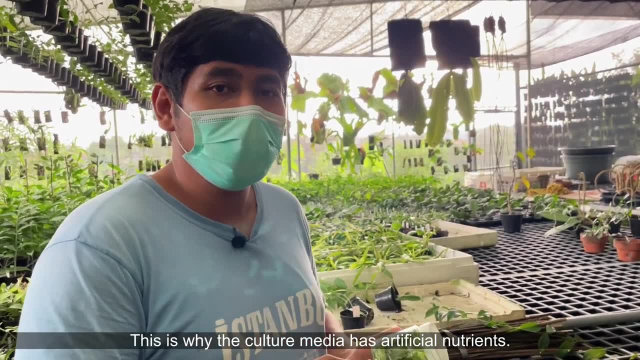 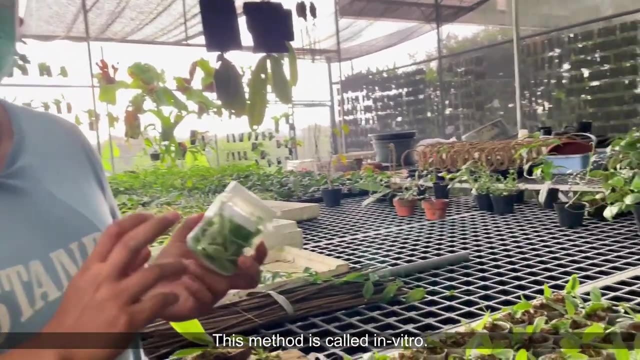 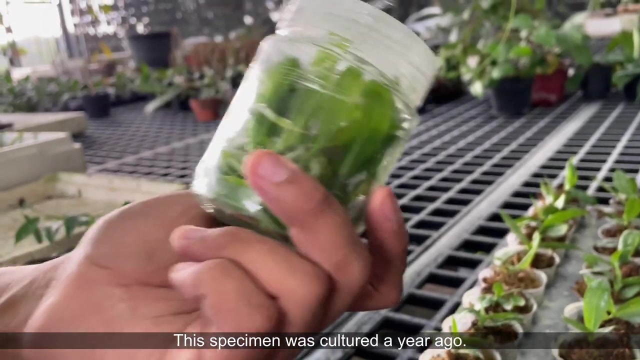 For the grape itself. it does not have a supply of food in the seed, so it needs artificial media to be able to grow. One way is with this in vitro technique. Here we can see that this is an old harvest from last year. 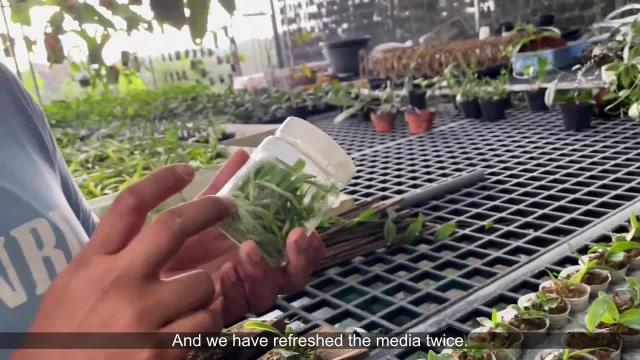 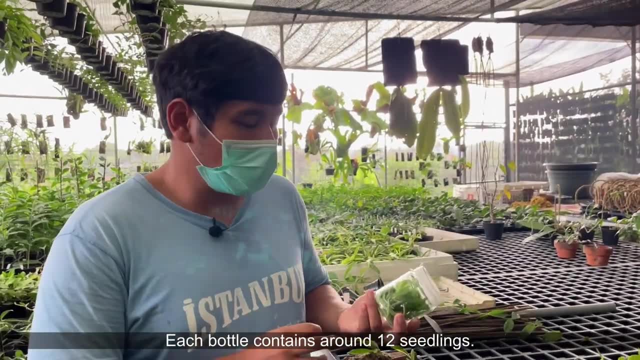 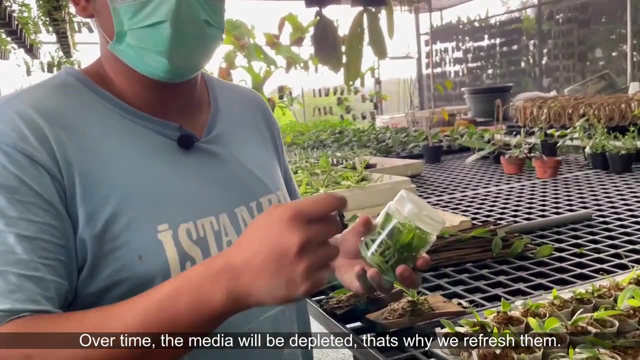 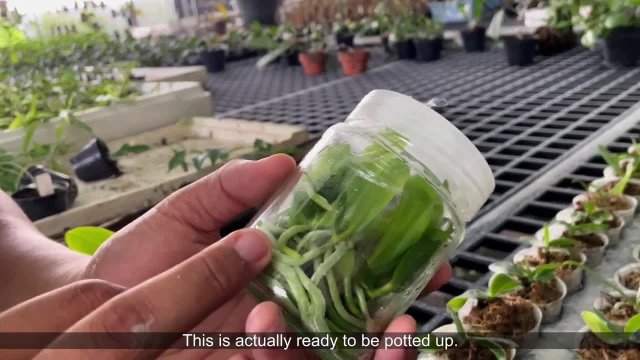 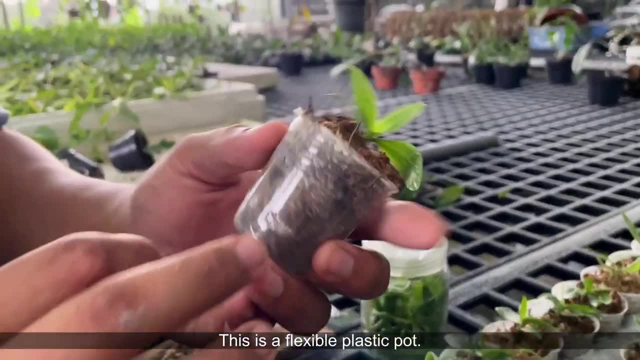 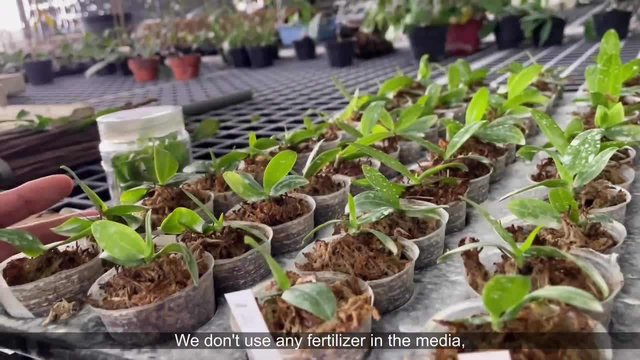 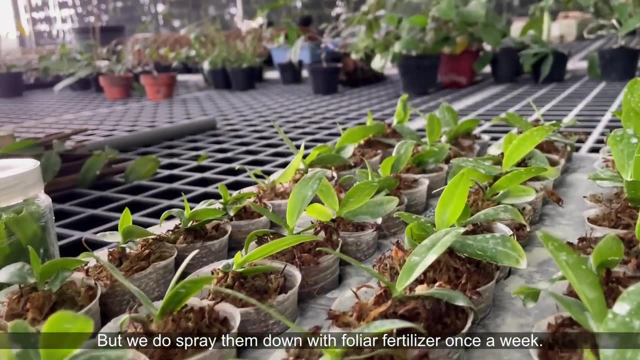 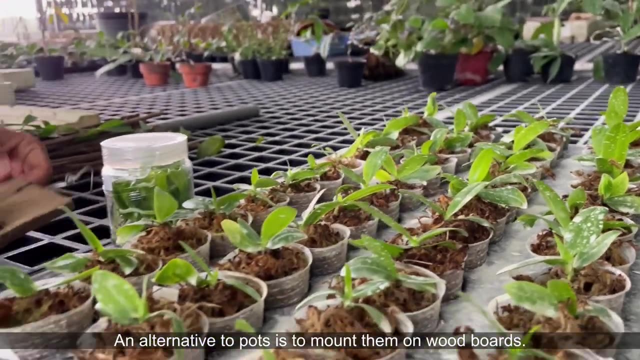 Do you use slow release here? No, we don't use any fertilizer. we just spray it once a week with leaf fertilizer. The other alternative: besides planting it in a pot, we can also plant it directly on a wooden board or a pachis board like this. 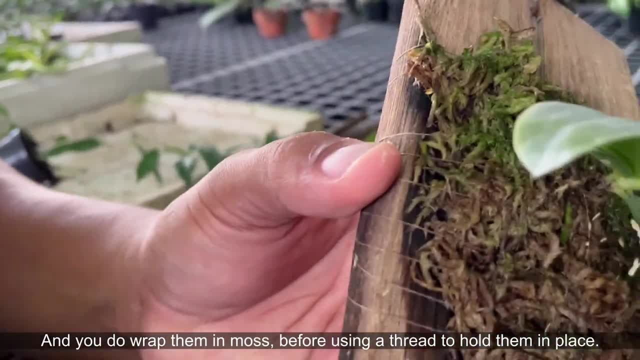 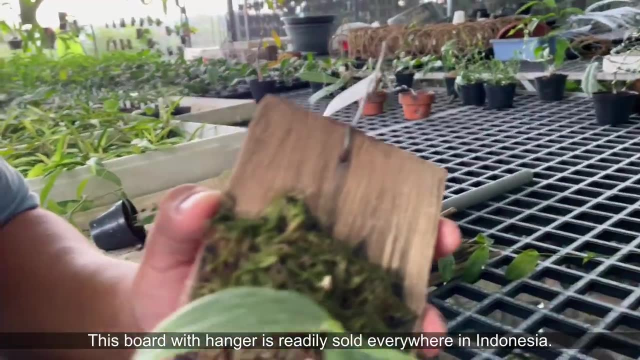 So it's the same as using moss. we just tie it up like this. We can buy it as it is right, Because in the online shop we can buy it as it is, But does the wood have to be of a specific type? 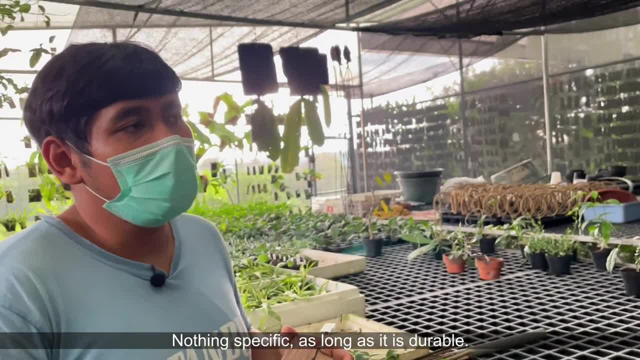 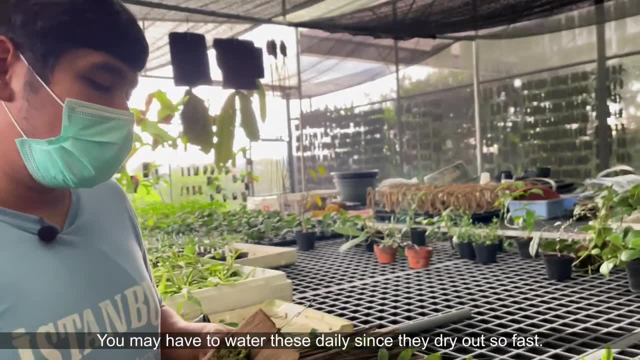 Actually there is no specific type. The longer it lasts, the better it is, so we don't need to transplant it. If we spray it more often, maybe every day, every one or two days- we can't spray it often, right? 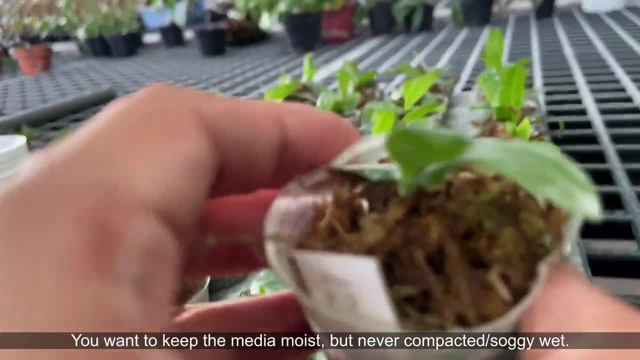 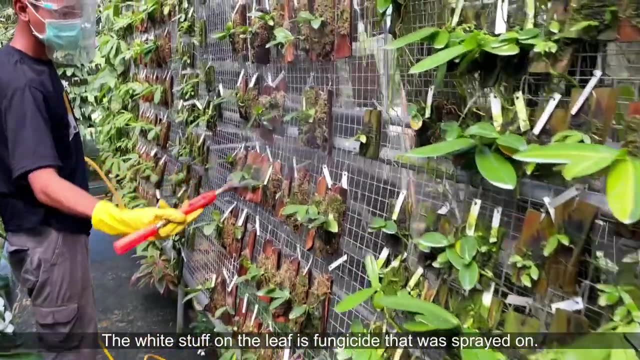 Yes, you can't spray it often, So if possible it should be moist, but don't let it be dirty. This one was just sprayed in the morning so it looks really dirty, And this one is anti-fungicide. the white ones on the leaves right. 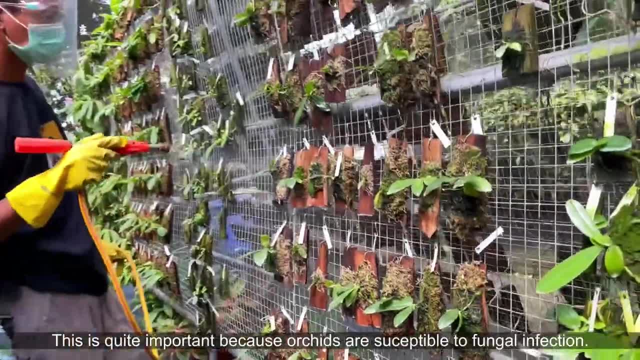 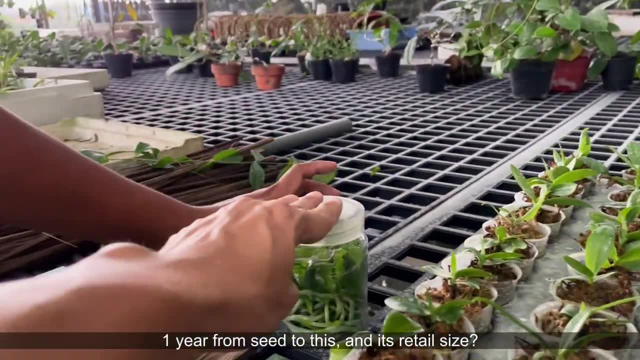 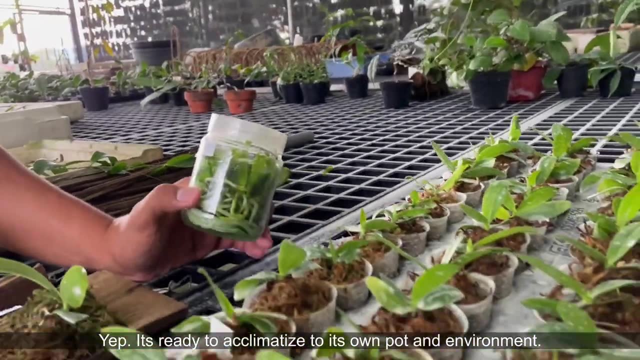 That's right. So it's important because it's easy for the leaves to rot, Especially in rainy season. So one year from the seed to here and this is already retail size, right? Yes, this is ready. The term is acclimatization. 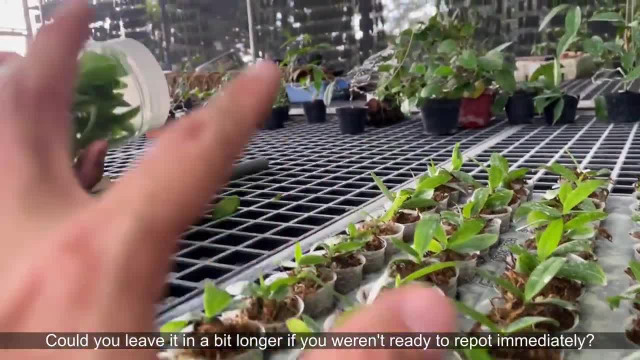 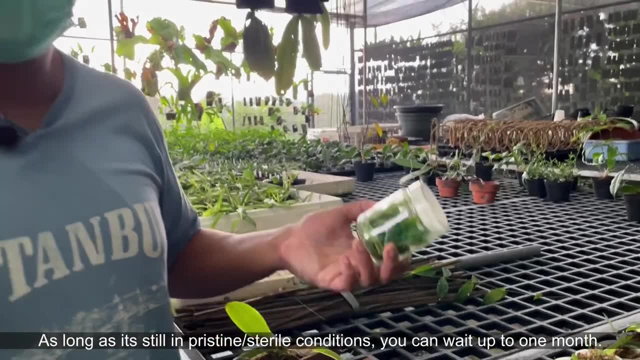 So if you buy it, it's ready to be transplanted? Yes, it's ready to be transplanted. If you don't want to transplant it, can you leave it inside? If the condition is still sterile, we can transplant it a month later. 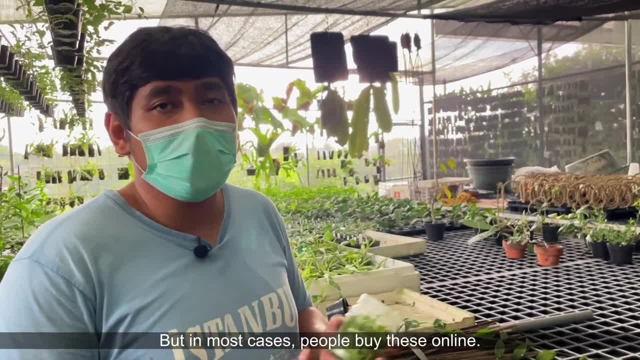 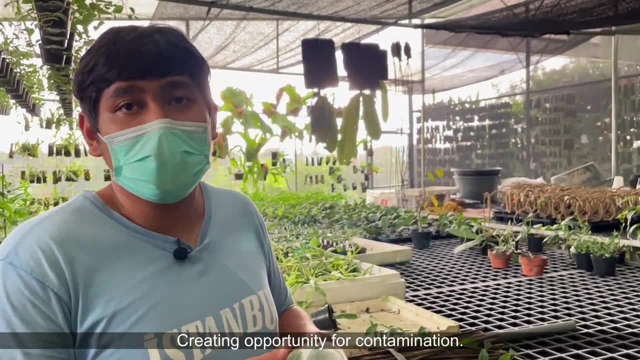 But sometimes when people order this, they say oh no. For example, when it's being delivered there's a mess, there's a possibility that it's contaminated, so it's better to get it acclimatized as soon as it's received. 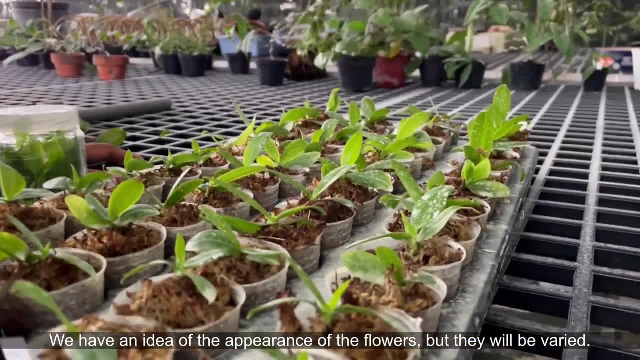 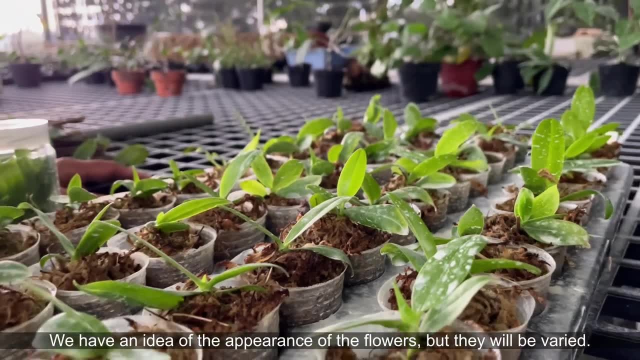 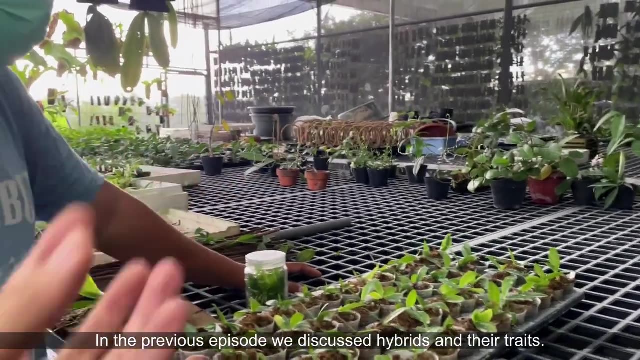 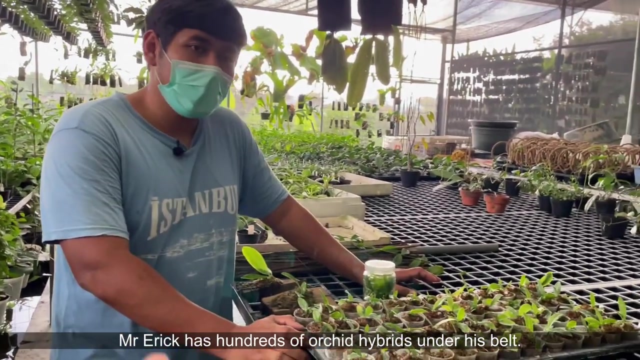 If this is the flower, we already know, but there will be a lot of variations, so it's still a mess. So in the next episode we're going to talk about hybrids that Pak Erik has already hybridized, because Pak Erik's background is hybridizing orchids. so stay tuned for the next episode when we talk about hybrids. 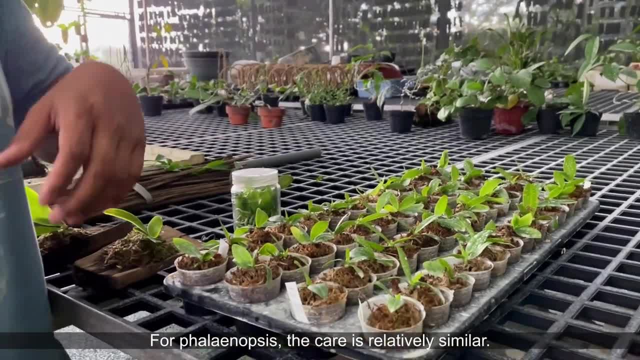 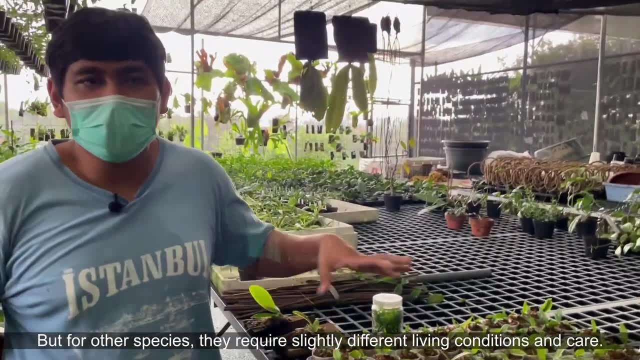 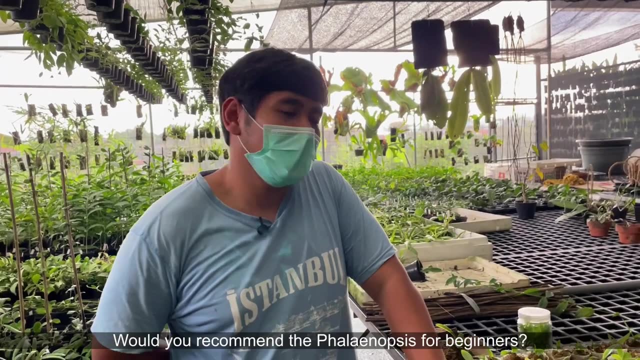 For Phalaenopsis it's more or less the same, but for other species it's different. So if we have too many species it's confusing. We have to adjust the environment accordingly. That's right, But for Phalaenopsis it's recommended, right. 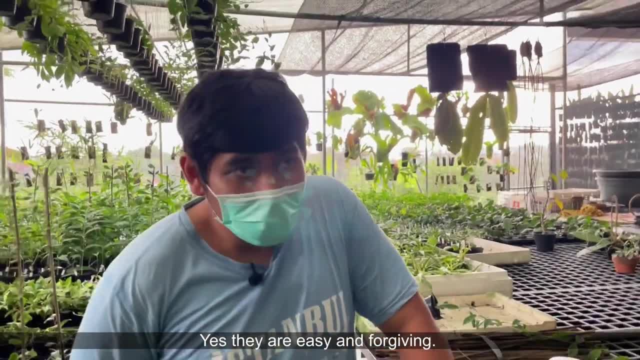 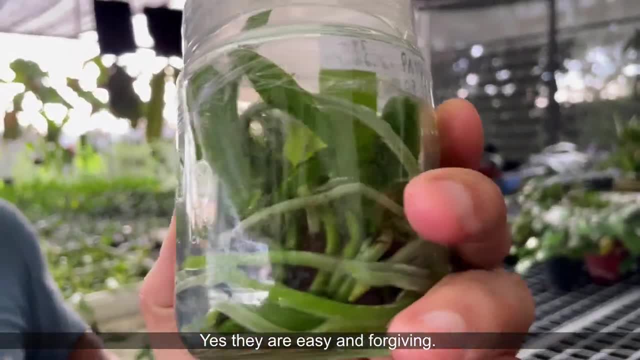 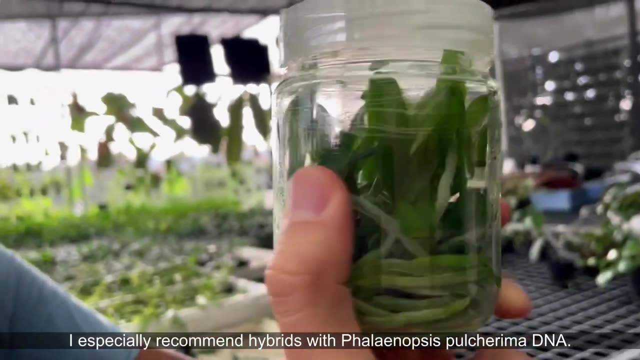 Actually, for beginners, it's pretty easy. right, It's pretty easy For the type that's usually for beginners. it needs to be durable. Well, that's better. Actually, we're looking for the one that has the blood of the month, which is called Phalaenopsis pulcherrima. 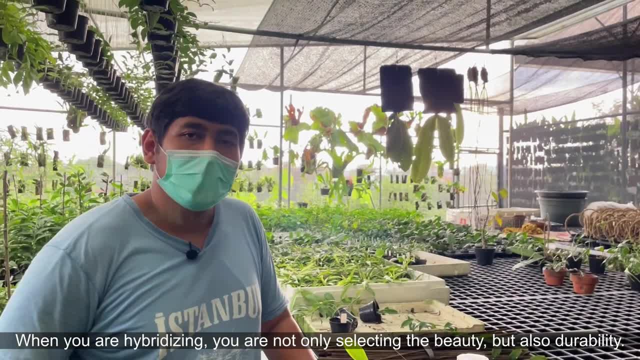 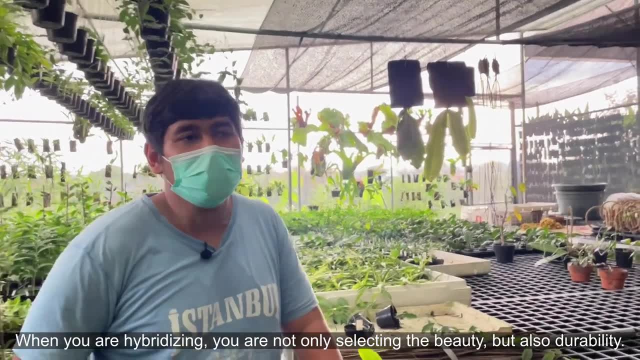 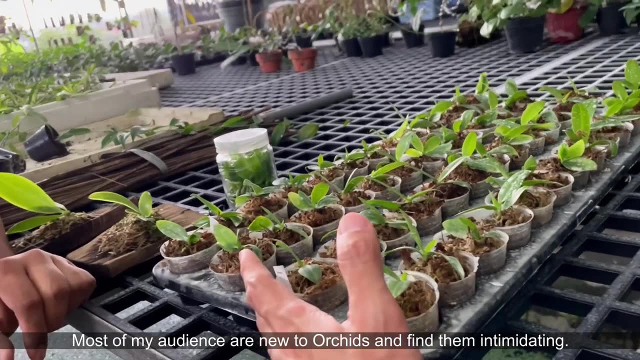 So when you hybridize, you don't just look at the character, but from the growth, right? Yes, So it's either easy or hard, fast or slow. Yes, usually the growth is very influential. Yes, Because many of our audience are still newbies and actually many of them comment that they are afraid of hybrids. 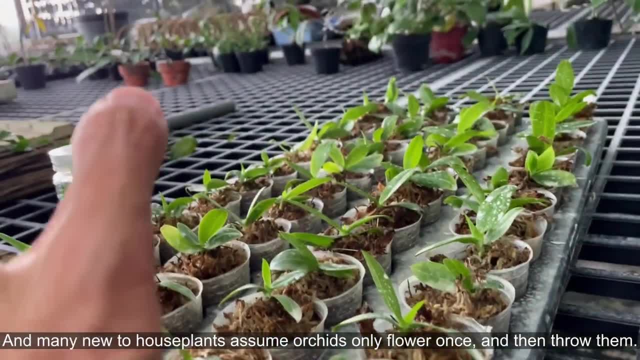 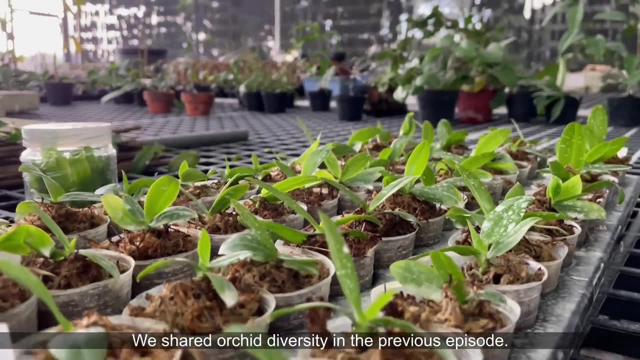 Because they often kill or see Phalaenopsis hybrids after one month, two months of flowering and then they throw it away. But actually they are very diverse. In the next episode we will discuss and give an example of how many flowers they are actually beautiful, beautiful and many that can be explored. 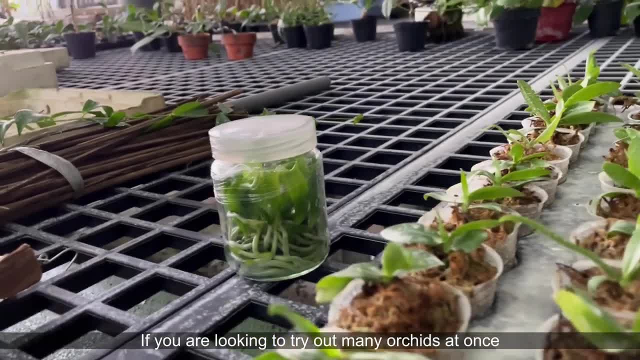 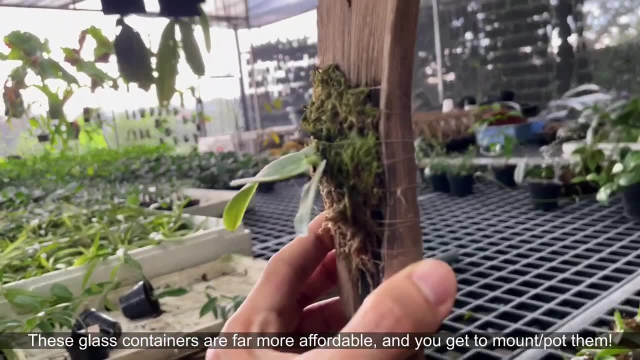 In this episode we will explore how to buy hybrids that can be said to be economical, but we can also enjoy what we have. We can plant it here. We can also plant it directly on the tree, right, The binding is a bit complicated. 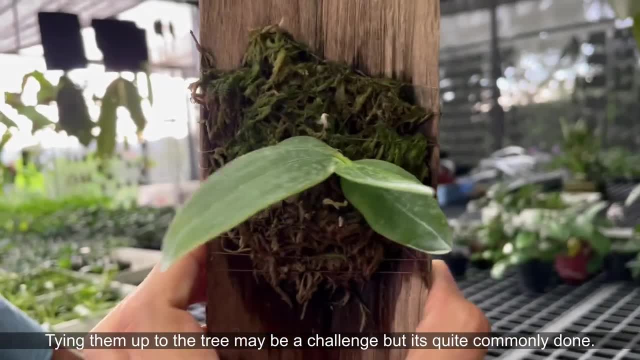 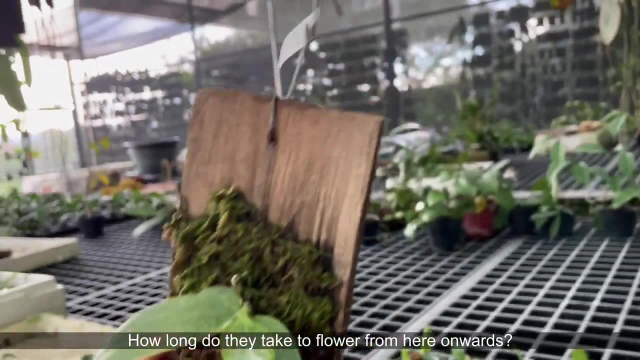 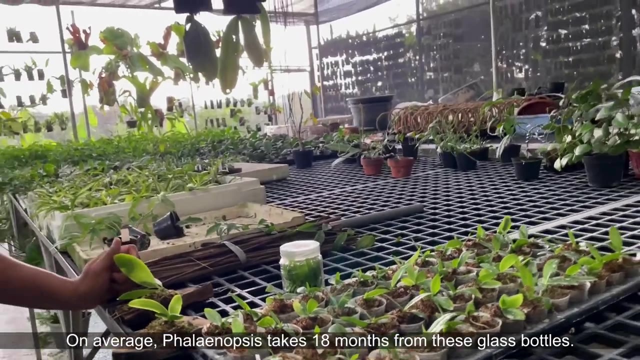 The binding is a bit complicated, But if it's just one bottle, it's fast too. Imagine if the tree is filled with this. It's all beautiful, Good, good, From here until it blooms. how long does it take? On average, the standard Phalaenopsis is about 18 months. 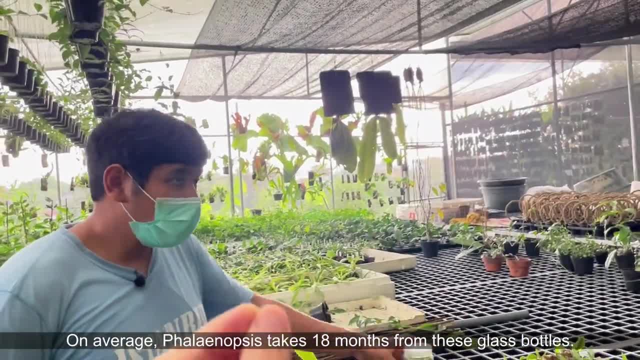 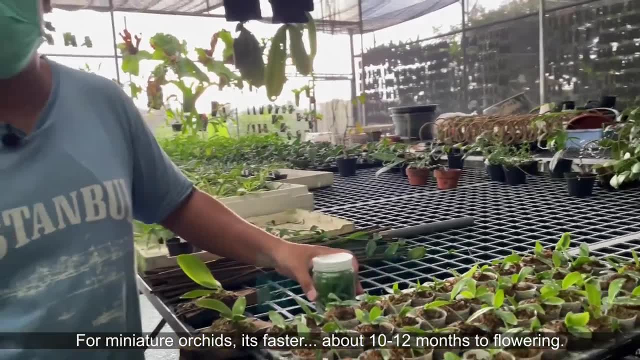 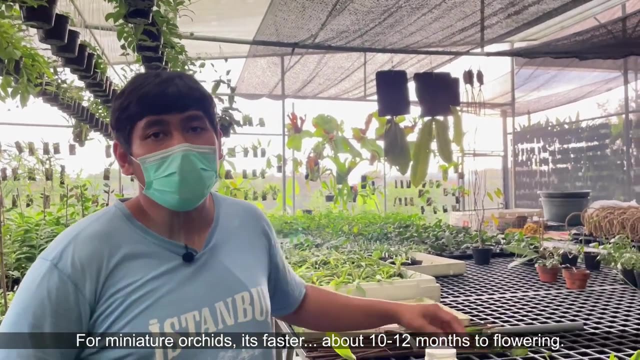 18 months From here or from the seed. From the seed that was acclaimed earlier, it's about 18 months. Well, it can also be more. For the types of miniatures it can usually be faster, Maybe only one year or 10 months. there are already some that can bloom. 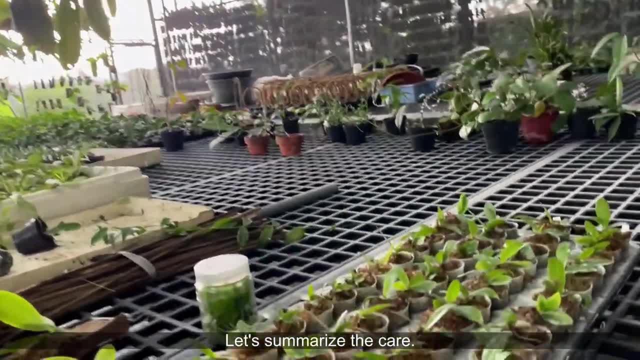 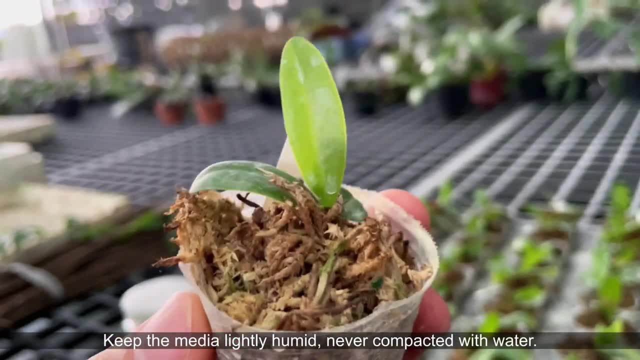 Nice, Okay, so quick care again. It's not too dry, but don't wait until it's dry. Don't wait until it's too dry, right? So it's still a bit moist, It's still a bit wet before it's dry. 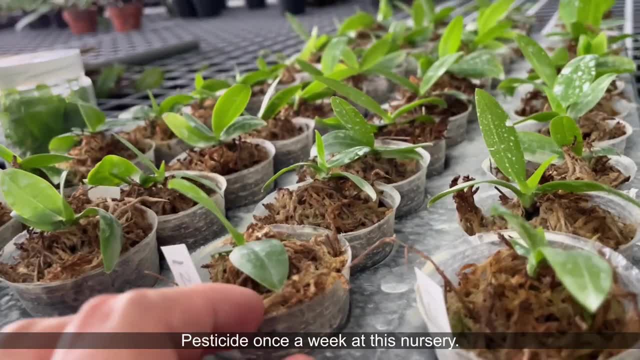 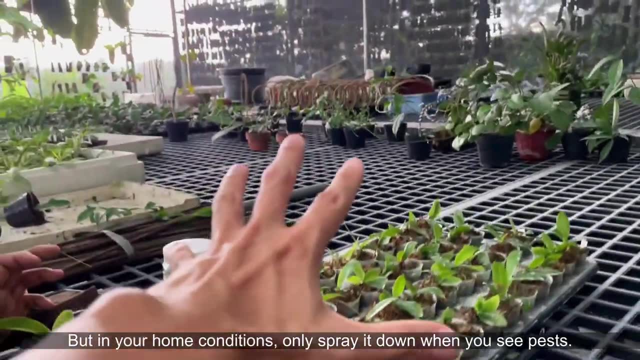 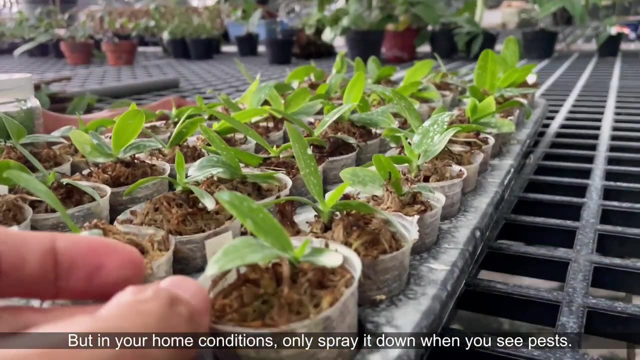 Okay, not fully dry. What about pesticides? Every 2-3 weeks? Once a week, usually, Because there are a lot of plants here, But at home do people sometimes need it? Actually, if there are not that many plants, just look at it. 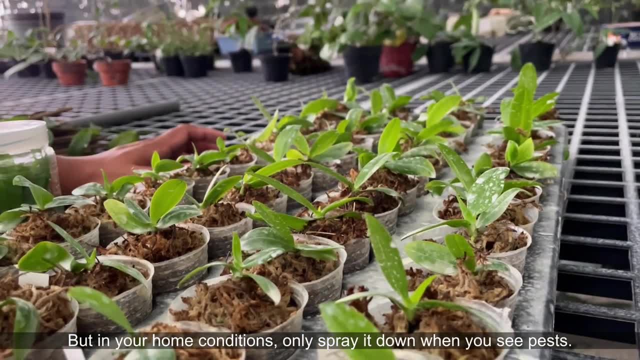 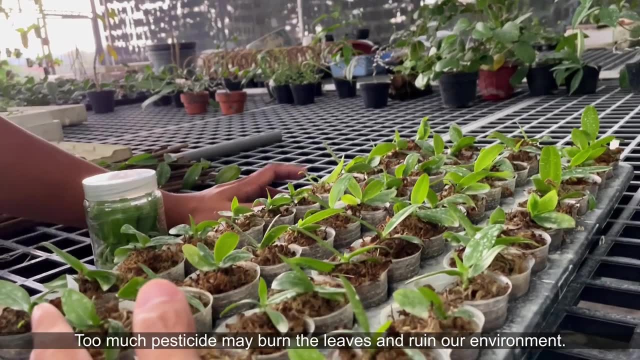 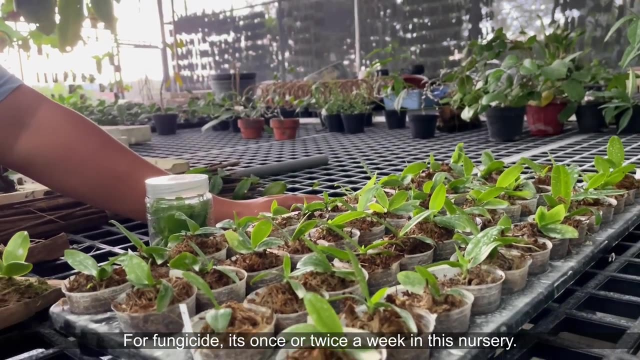 If there are signs, then give it a pesticide, Because we also want to avoid too many pesticides. it can also burn the plants and damage our environment, Right, But anti-fungi, anti-fungus Recommend, right, Can it be often? 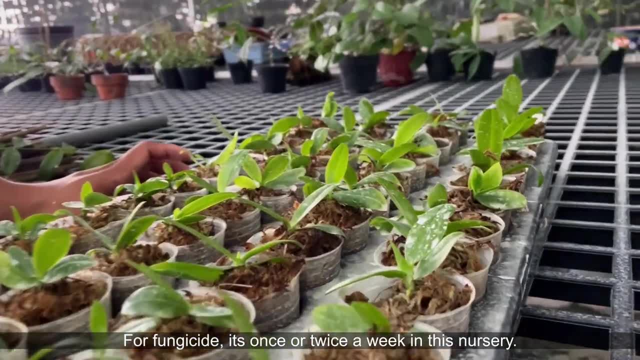 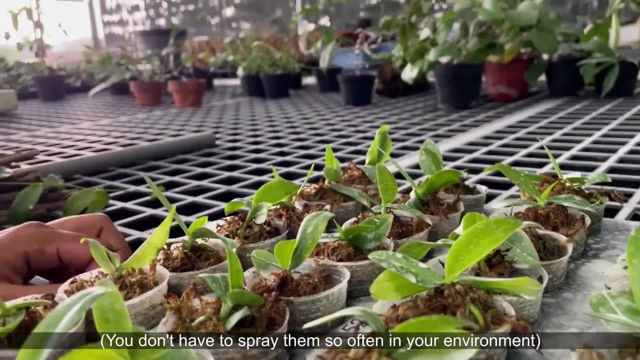 If it's here, it's most often once a week. Sometimes, if there is no attack, this is because of the rainy season. it's twice a week. Okay, so it's according to your needs. What about fertilizer, If it's fertilizer? 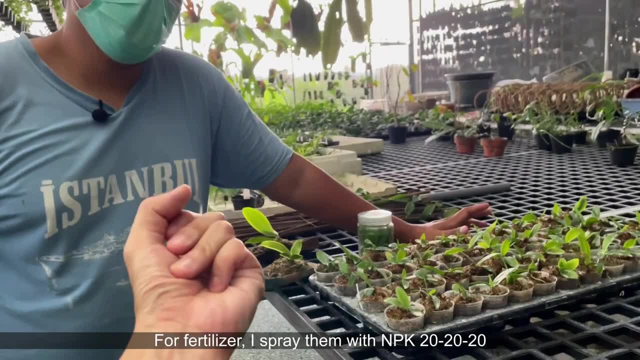 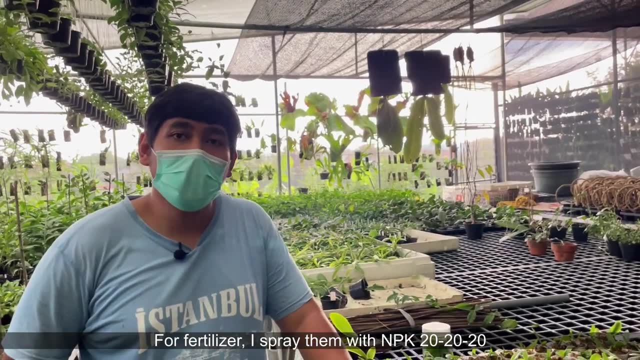 now once a week, Fertilizer or just grow more, Just that kind. if I use it, the NPK fertilizer is 20-20-20.. Okay, balance mix water, dilute spray: Yes, the concentration. 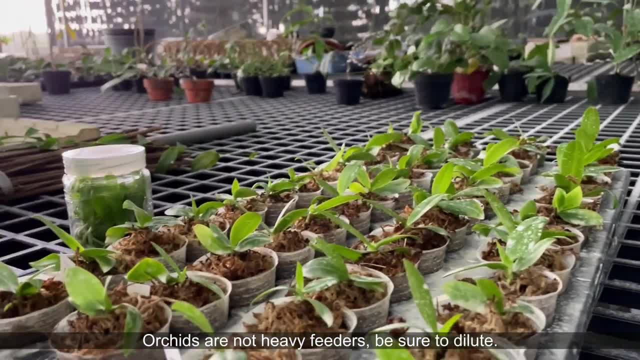 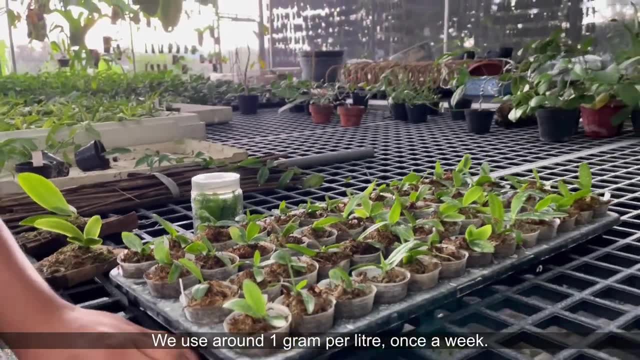 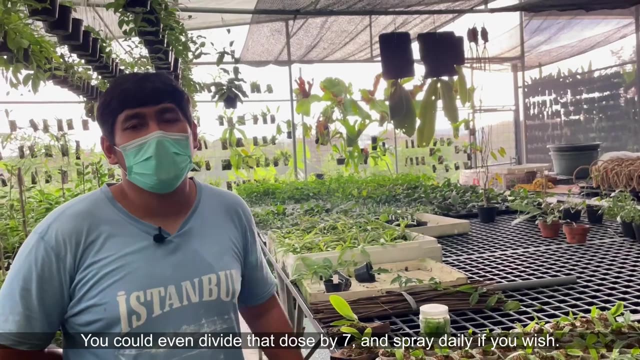 because this fertilizer doesn't really need a lot of nutrition, so the concentration doesn't have to be a lot, Usually 1 gram per liter or, if you want to dilute it more, for example 1.8 doses. we can spray it every day, for example. 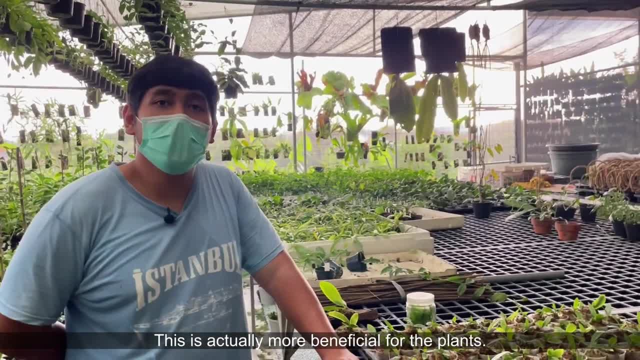 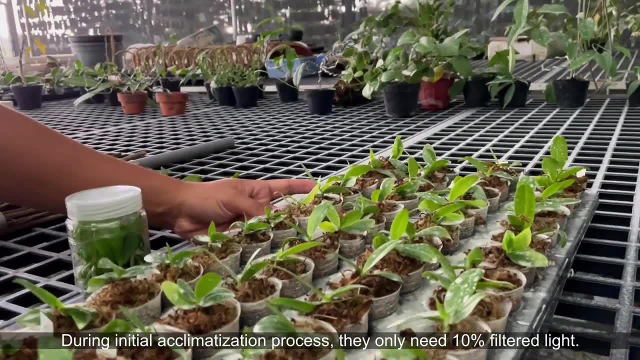 But it's better often. but the dosage is a bit reduced, That's right. it's actually better like that And it's bright, but don't direct sunlight. If it's Phalaenopsis, if it's just acclimatized, it usually only. 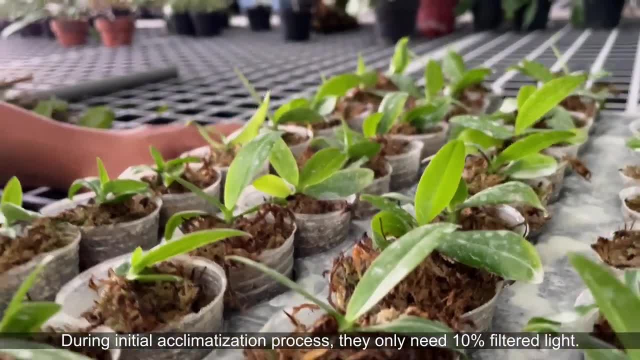 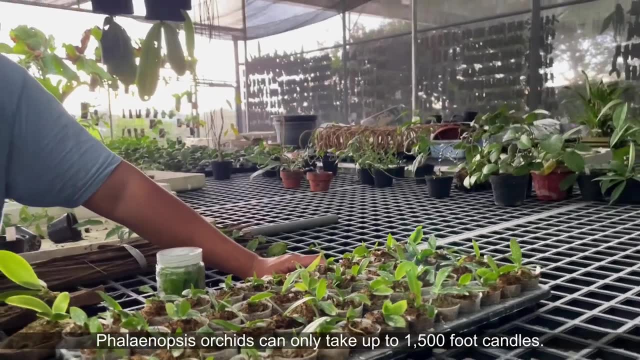 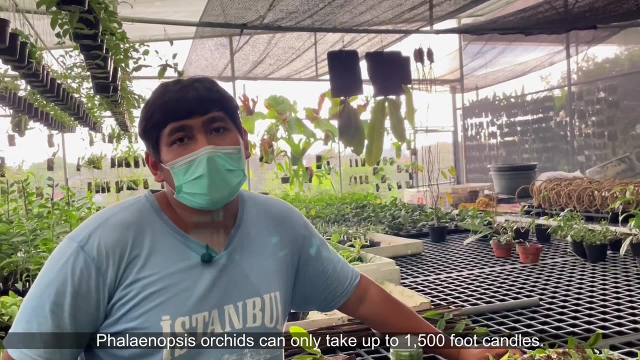 needs 10% light, Just like that. Just like that. So the highest- if in food candle the monthly yield is only the highest- is 1,500 food candle Which he can accept, Which he can accept, Wow, so it means I have brightness. 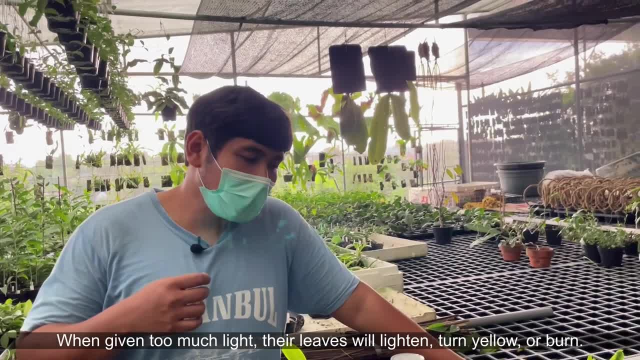 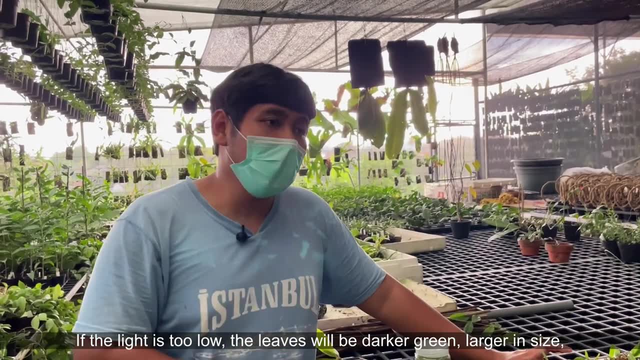 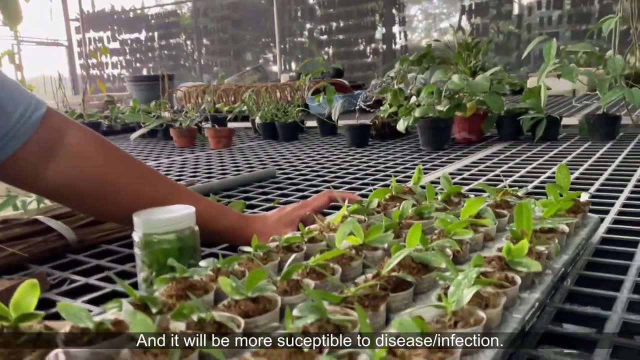 Yes, usually if it's too bright it will turn yellow or sunburn burn, Or if it's too dark there's a problem. The leaves will also be too far away and the leaves are big, Then it's easy to get sick. 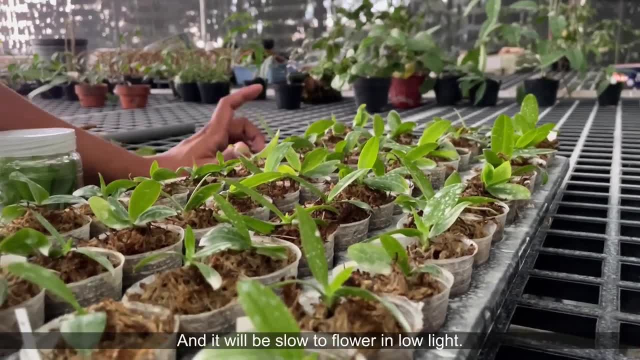 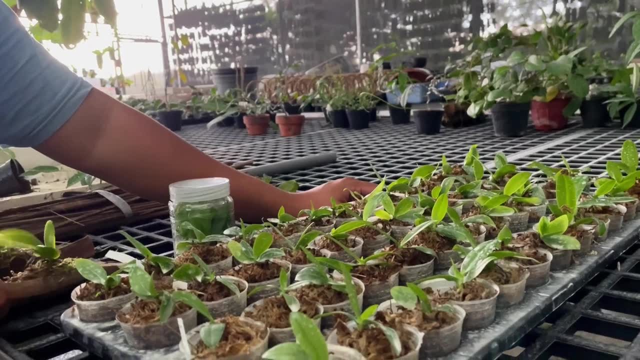 But the flowering is also slow. If it's too dark, the flowering is too long. If it's too bright, the flowering is faster. Okay, I guess that's it for today's episode. This is an interesting mini project. I hope that you can pick one up. 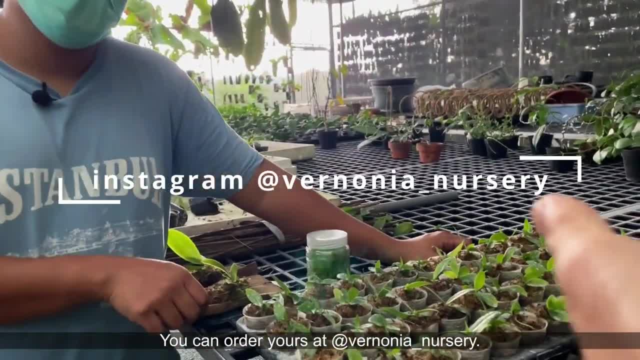 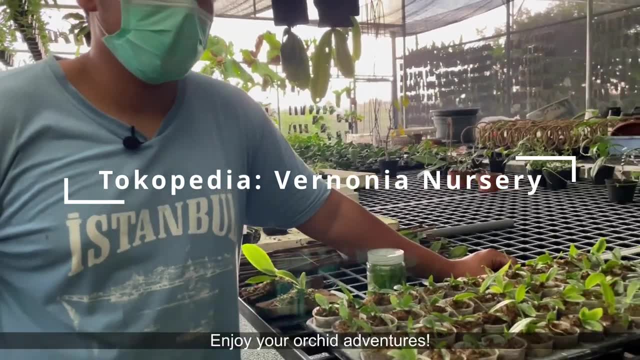 Of course, you can buy this at Vernonia Nursery. There's Tokopedia, right? Yes, there's Tokopedia. There's a link below. Please make an adventure. It's not expensive and it's enjoyable. I will try myself as well. 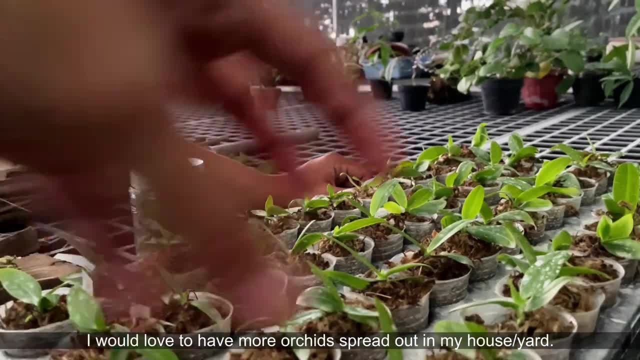 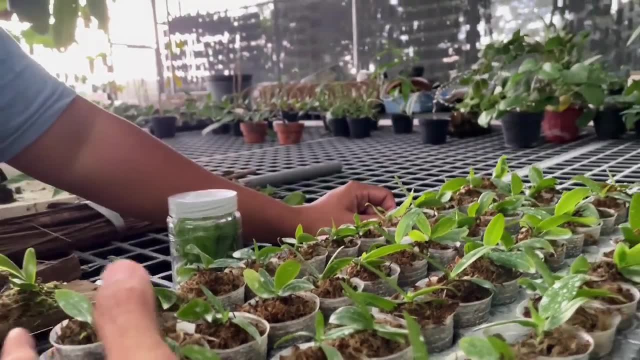 Because I like it when there's orchids near my house. The flowers are really beautiful and the leaves are also beautiful. Thank you so much for the share. I'm at botanist on Instagram If you want to DM me on any questions.